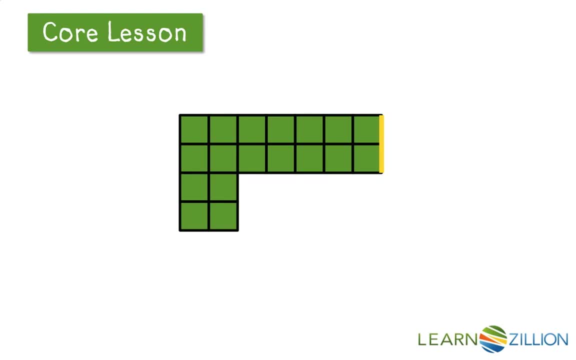 know when one side length stops and when another starts. I am highlighting the side lengths of this polygon To find the perimeter of the polygon. I do the same exact thing I did with a regular shape, With a regular square rectangle: I find the side lengths and I add them up. I can find the side. 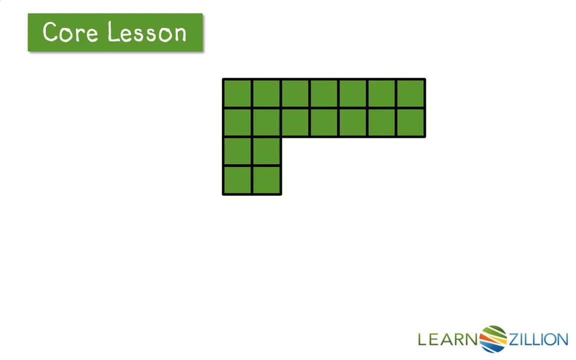 lengths by counting the squares along each length. So there's one, two, three, four, five, six, seven, seven units on this side: 1, 2, 3, 4 units on this side: 1, 2 units on this side. 1, 2 units on this side. 1, 2, 3, 4, 5 units on this side and 1, 2 units on this side. now, all now I. 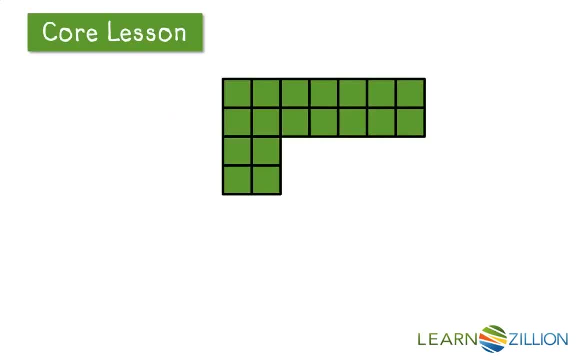 have all of my side lengths so I can write a number sentence and find the perimeter. so 7 plus 4 plus 2 plus 2 plus 5 plus 2. so 2 plus 2 plus 2 is 6, 6 plus 4 is 10, 10 plus 5 is 15, 15 plus 7 is 22. so the perimeter of this shape is 22. 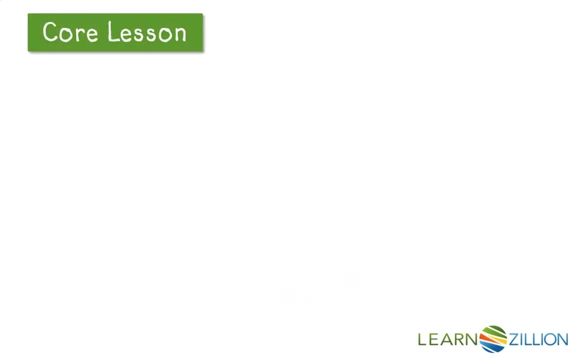 units. let's go back to that first point and we'll move on to the second point and we're going to go back to the polygon we saw and let's find the perimeter. Again, I will find the side lengths by counting the squares that make up the length. So that's one, one, two. 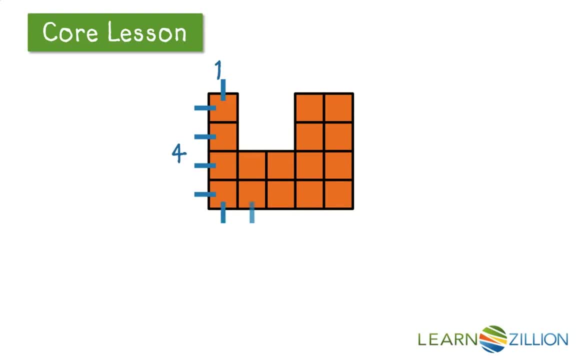 three, four, one, two, three, four, five, one, two, three, four, one, two, one, two, one two and one two. So now I have all of my side lengths. I'm going to write my number. 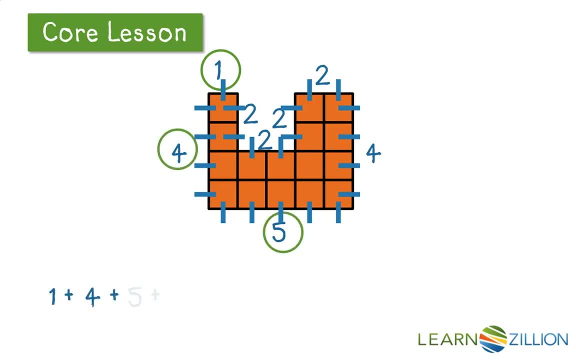